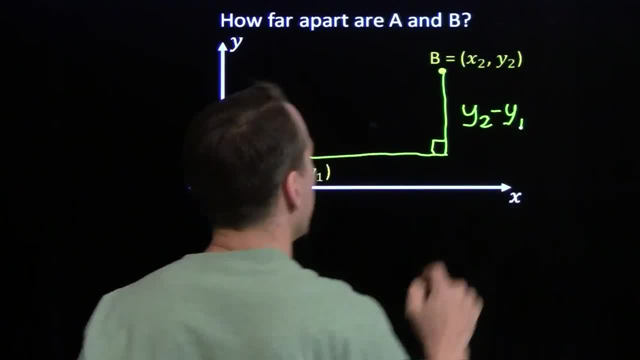 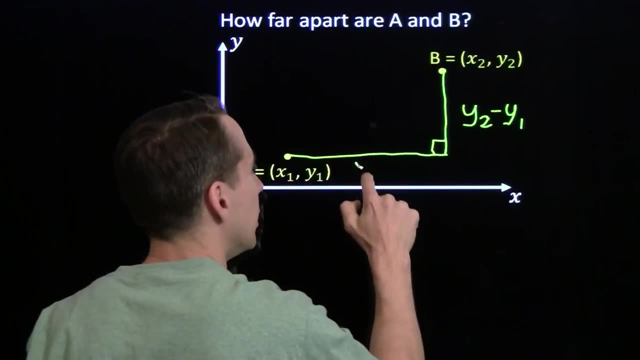 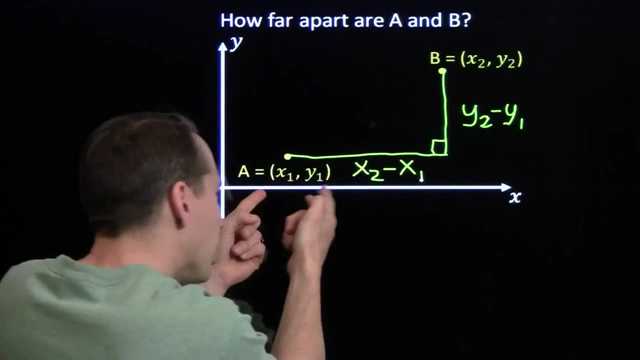 This is Y2 minus Y1.. And then this right here: that's how far we're going left to right. That's the difference in the X coordinates: X2 minus X1.. Now we see why we're putting these little subscripts here and why we call these points X1, Y1, X2.. 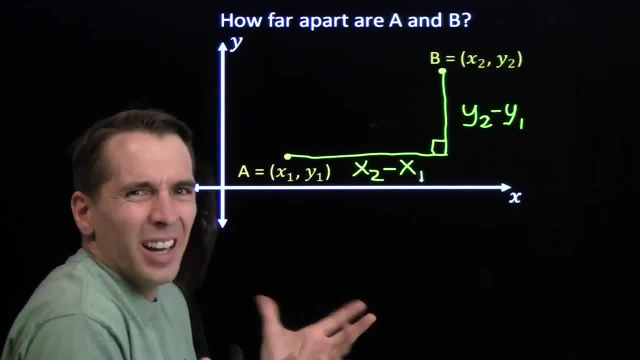 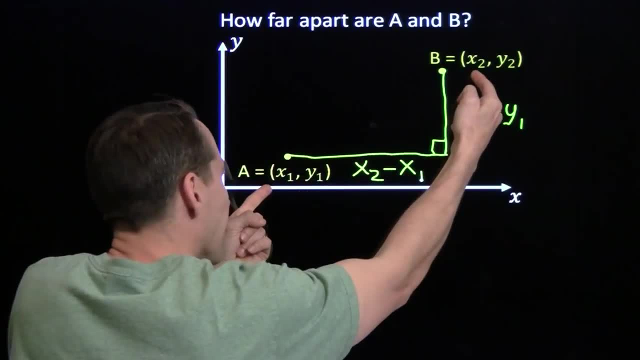 If we called them AB CD, that'd be a little confusing. You wouldn't be able to see that these are both X coordinates. These are both Y coordinates, But here we can see that X1 and X2 are obviously X coordinates. That's what the X is for. 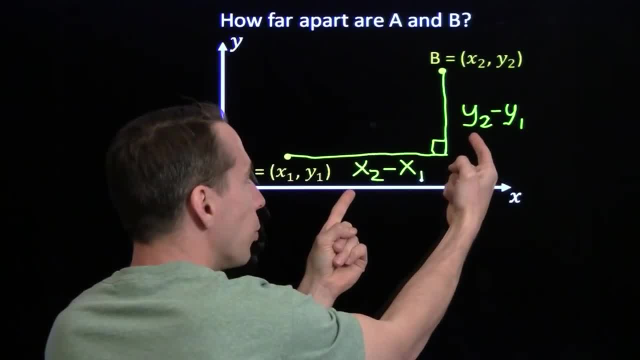 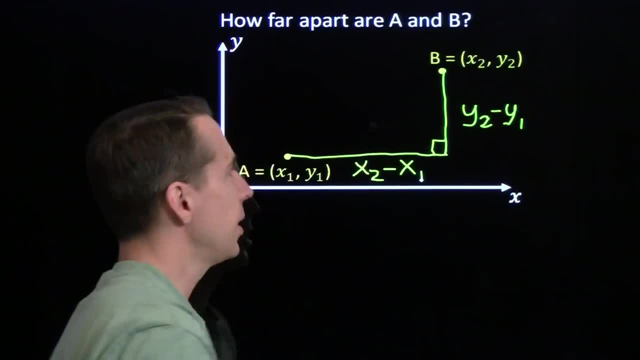 And the twos, the twos down here they tell us that these two both go with the same point. These two both go with the same point because they're both ones. That's why it's nice to use these little subscript things here instead of using just four different letters. 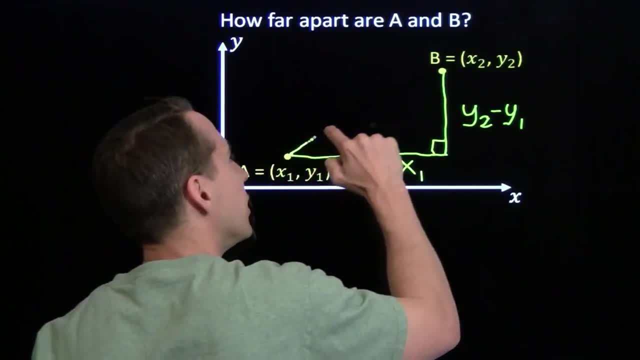 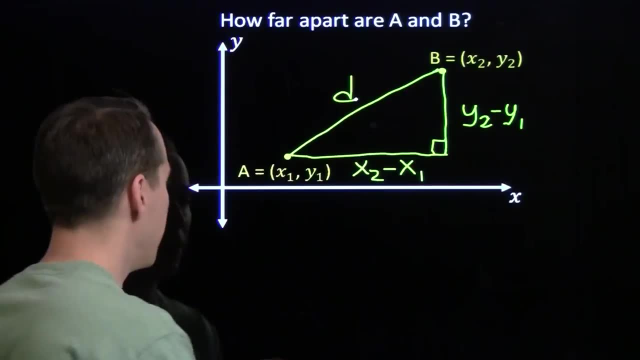 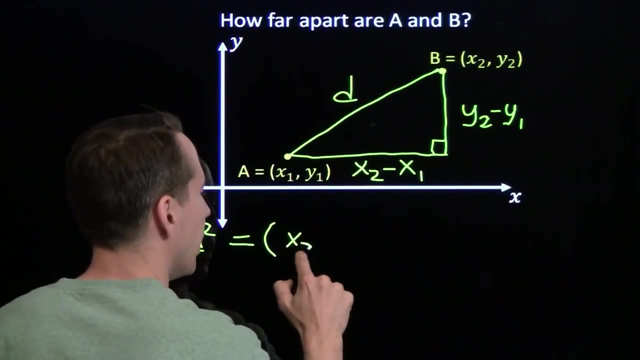 Now we've got the legs of our right triangle. We can figure out the hypotenuse in terms of all these X's and Y's. So let's call that D. We break out the Pythagorean theorem And we have D squared, that's. the hypotenuse equals the sum of the squares of the legs. 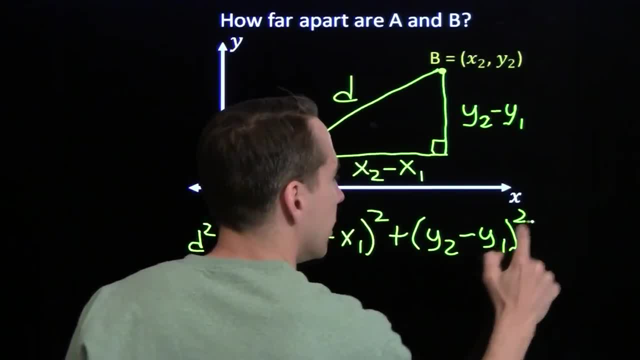 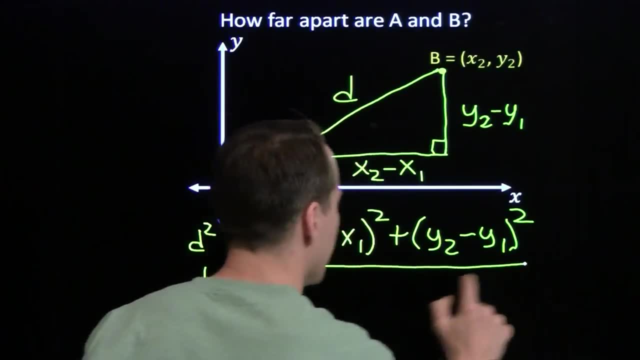 And that's all there is to it. Now, some people like to take the square root of this, So we just have D. Let's give this a fancy name. They call it the distance formula. Okay, it's not that fancy, It's not even that clever. 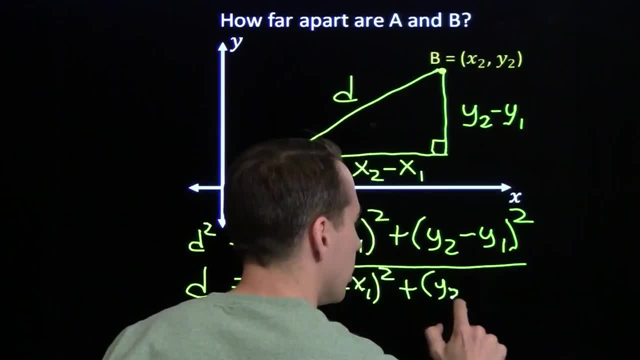 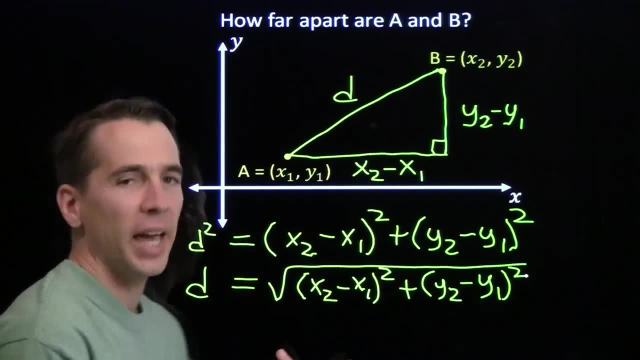 And you know what? It's not even something new. I don't think of this as the distance formula, I think of this as the Pythagorean theorem, And if you just think of this as the Pythagorean theorem, well then you don't really have anything new to memorize here. 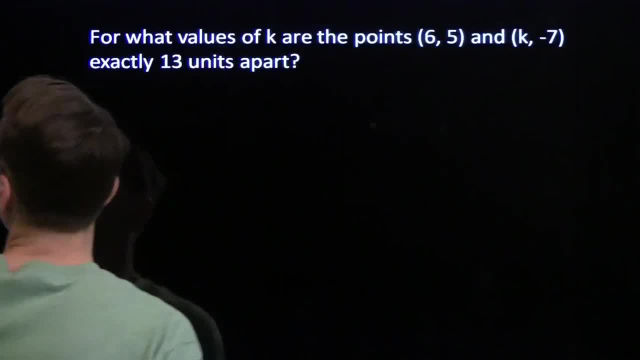 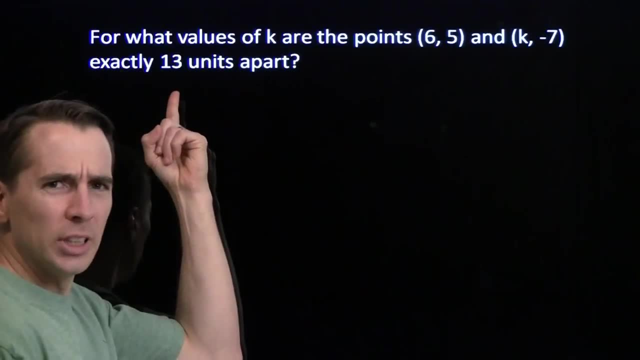 You already know this. Now let's try putting this to work. Oh, okay, let's see The values of K. are these two points Exactly 13 units apart? Well, we know how to figure out how far apart these two are. 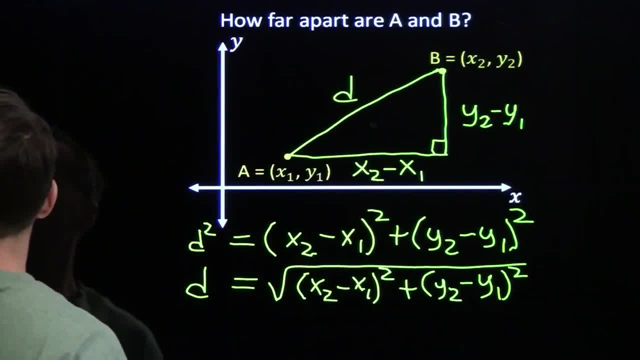 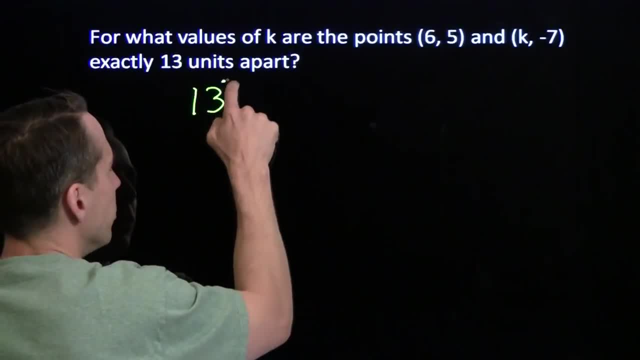 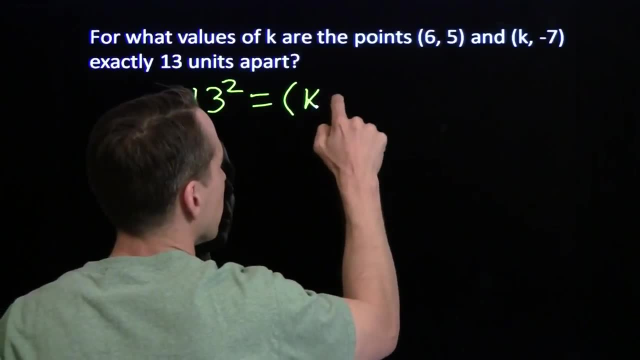 We're breaking out our Pythagorean theorem relationship right here. We know the distance between them is 13 units, So that's kind of the hypotenuse of our right triangle And that's equal to the sum of the squares of the difference of the X coordinates.